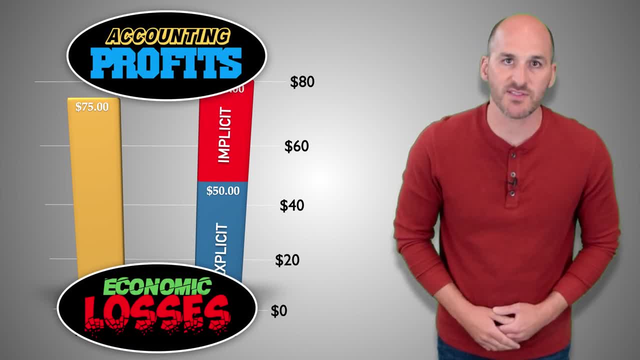 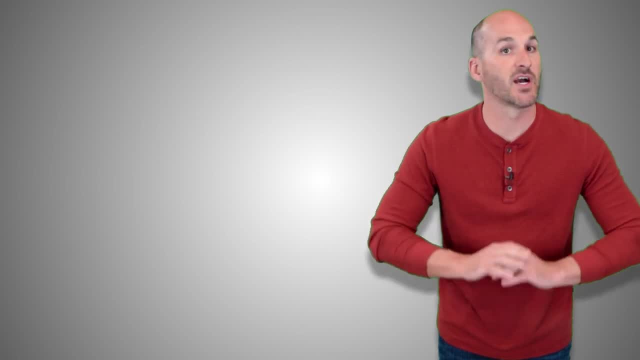 tr. República Libertad ger�도 de Fuerzappe. This means that they're earning accounting profit, but not enough to cover their economic capital products. accounting profits but taking economic losses at the same time. In economics we cut through the confusion and make things simple, because all costs are. 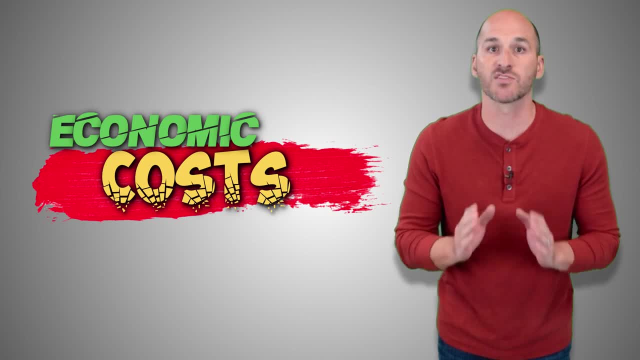 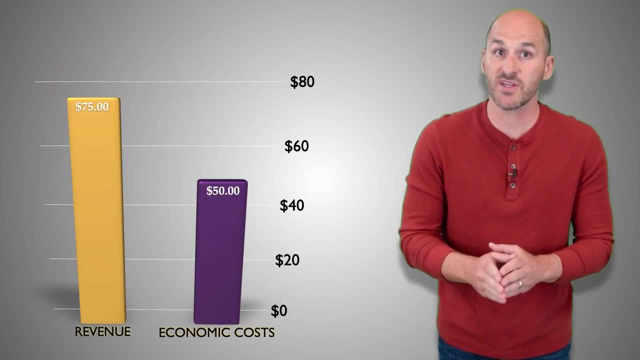 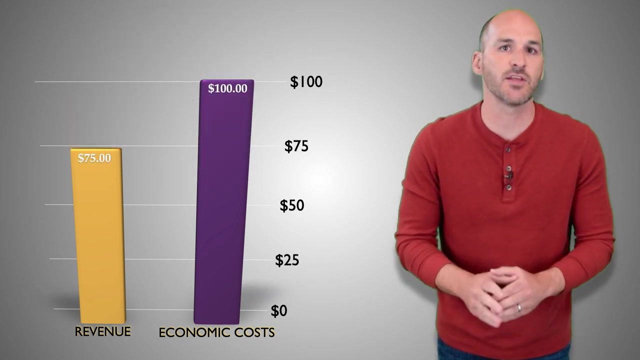 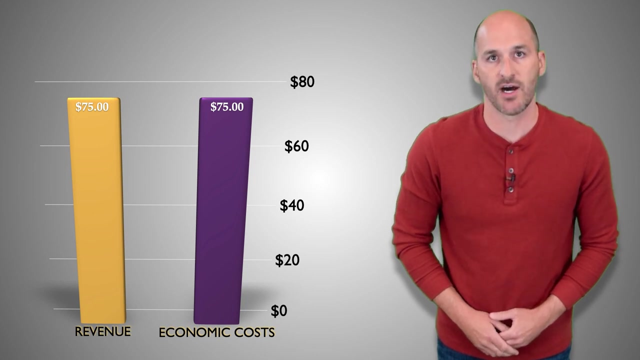 economic costs. Any and all costs of production from here on out include both explicit and implicit costs. If revenue exceeds economic costs, the firm is earning economic profits. If economic costs exceed revenue, the firm is taking economic losses. And if revenue equals economic costs, the firm is breaking even. When producing output, firms face several different types of production costs. Fixed costs are the wages and rents of the fixed resources used during the production process. These costs do not change with the amount of output produced and they can include rents on land or on land. 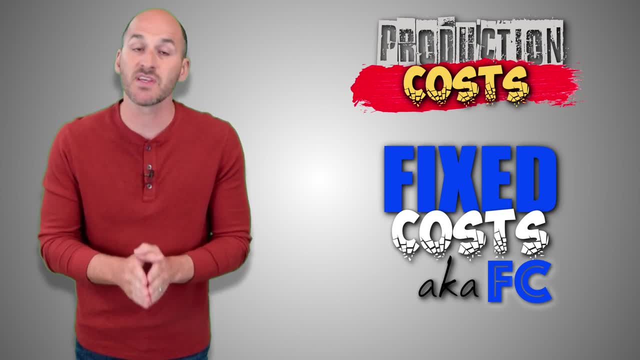 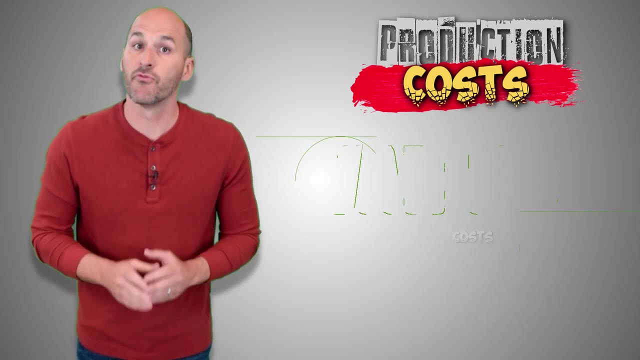 Interest payments on loans, as well as insurance and business licensing. Fixed costs are often referred to as overhead costs because they must be paid regardless of production level and sometimes even before production begins. Variable costs are the wages and rents of variable resources used during the production. 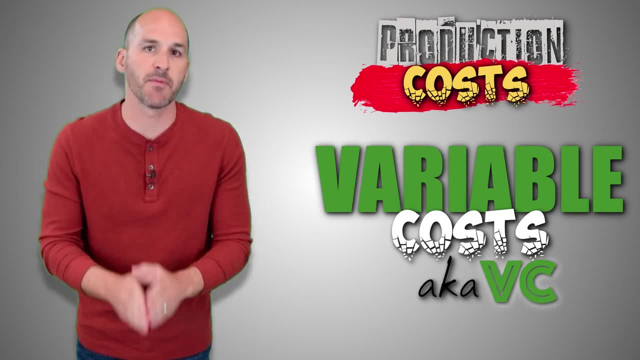 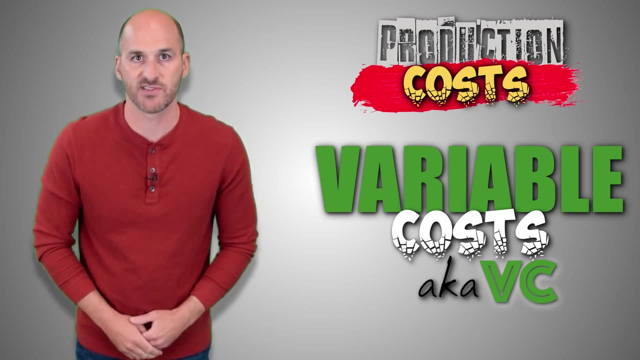 process. These costs do change with the amount of output produced. When the firm produces more output, it faces higher variable costs. When the firm produces less output, it faces lower variable costs. Variable costs include hourly wages paid to workers, as well as rents paid for electricity. 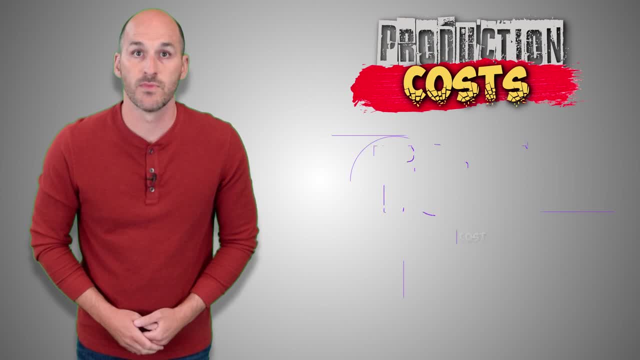 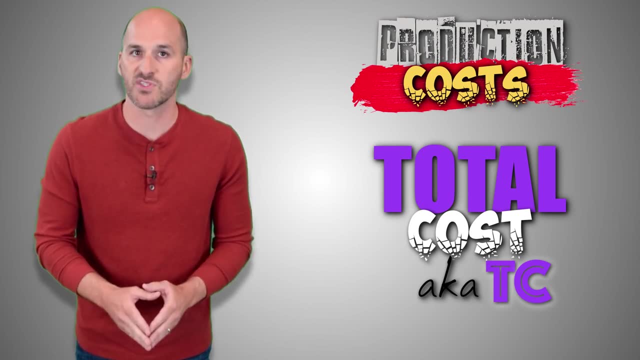 capital, equipment and raw materials. Total cost is the sum of the variable costs and the fixed costs of production. The more output produced, the higher total costs are to firms, because variable costs increase as production increases. The less output produced, the lower total costs are to the firm, because variable costs. 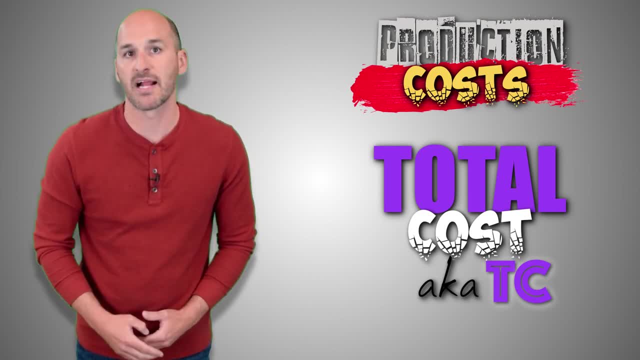 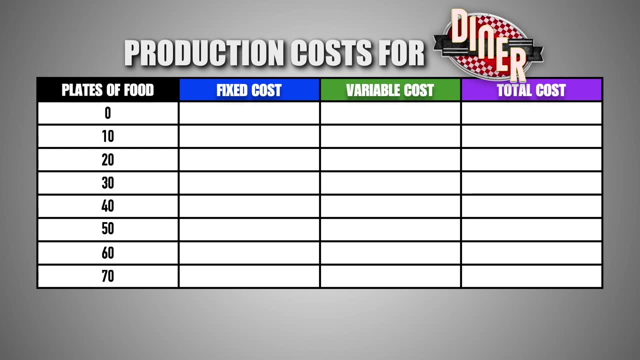 decrease as production decreases. Let's practice: Suppose an entrepreneur sets out to start a small diner in your hometown. To get started, the business owner is going to have to pay overhead costs on several fixed resources. Before opening his doors or even producing a single plate of food, he has to pay rent. 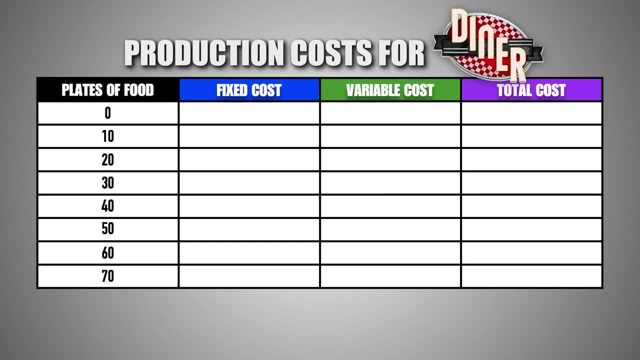 on his store, purchase fire insurance and pay for several required business licenses. These overhead costs add up to $100 in fixed costs for the firm before the doors have even opened or production has even begun, Because fixed costs remain constant and do not change with the quantity of output produced. 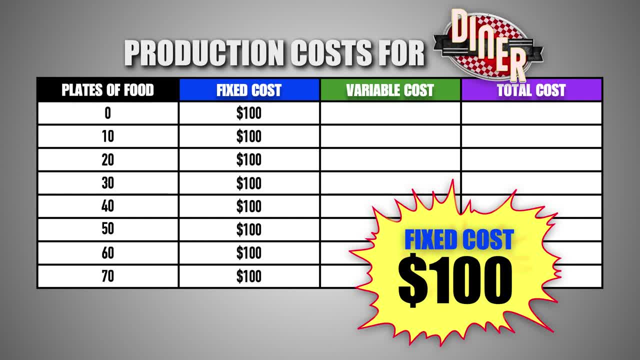 the firm will face this $100 fixed cost of production, no matter how much food they produce Now. in order to begin production, the firm will have to pay $100 in fixed costs for the store. The store owner has to combine several variable inputs, including labor, electricity, refrigerators. 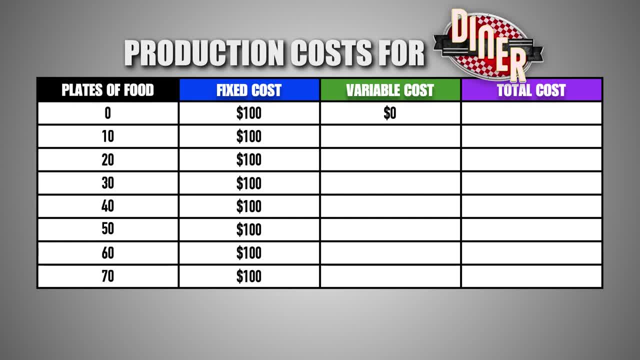 cooktops and other equipment. When combining the wages and rents of the labor and capital required to produce the first 10 plates of food, the store owner will face a variable cost of $80.. However, as output increases, the owner will have to hire more workers and rent more equipment. 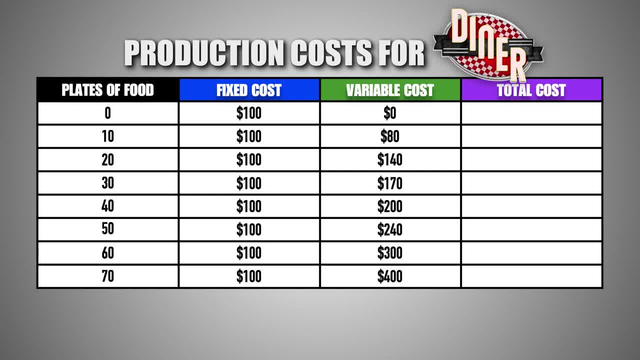 meaning that the variable costs of food will increase. The total cost of production will increase as production increases. From here we can calculate the total cost of production for the diner by adding the fixed cost of production to the variable cost of production at every output level. 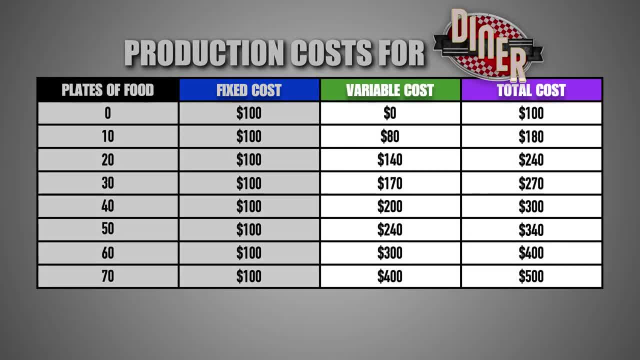 Notice that fixed costs remain constant at every output level, while variable costs and total costs increase as output increases. Also, notice that the difference between the total cost and variable cost of production at each output level is the sum of fixed production costs for the firm. 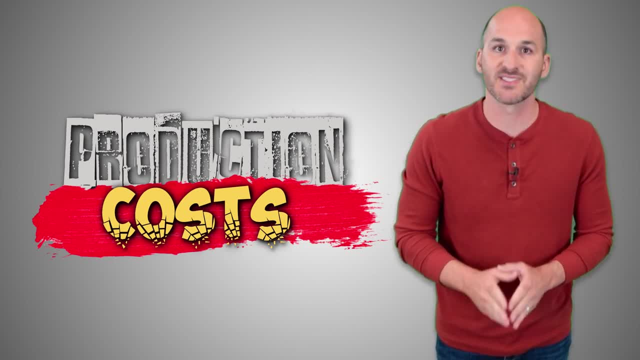 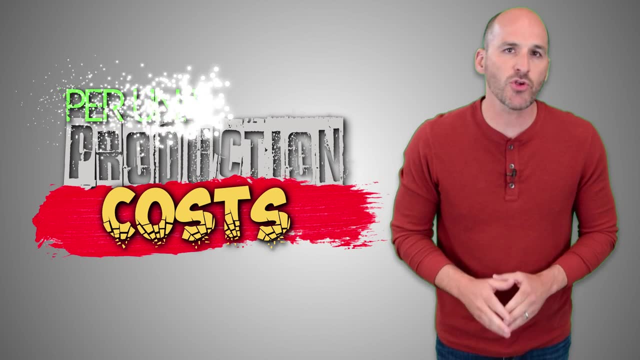 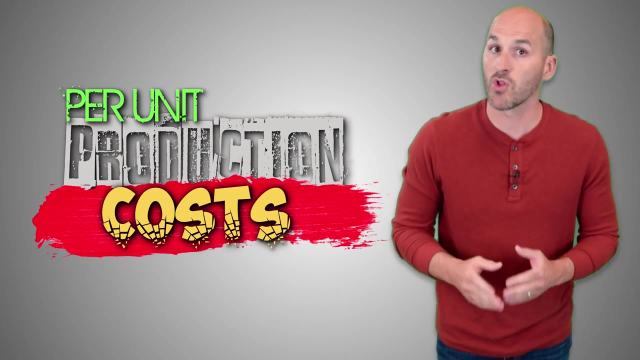 Because firms are seeking to maximize profits, it is important for firms to gauge the fixed, variable and total costs attributed to each unit that they produce. These per-unit production costs help firms decide the total quantity of output they should produce, as well as the profit earned or losses taken per unit of output. 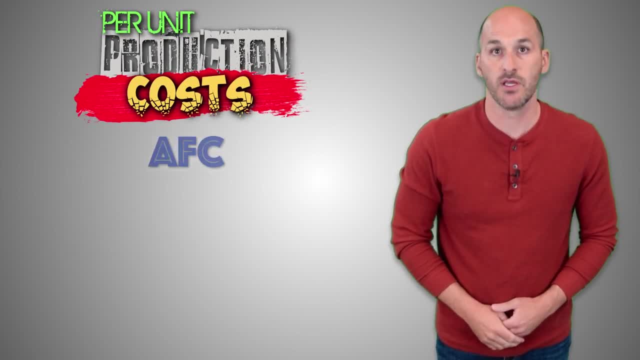 There are four different types of per-unit production costs. The first is the fixed cost of production, which is the total cost of production of the offering firm. The second type of fixed costs is the fixed cost of production, which haben a corporate firm net average of production per unit of output produced. To compare the fixed costs between fixed and tractor production, you simply need to take the fixed costs of production and divide them by total product Average variable costs. tell the firm the variable costs of production per unit of output produced. To calculate the average variable cost per unit, we simply need to take the variable. 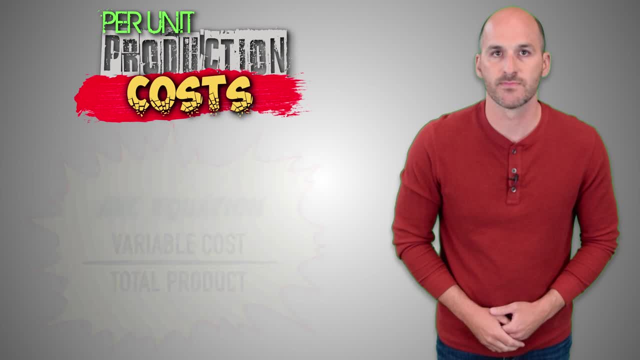 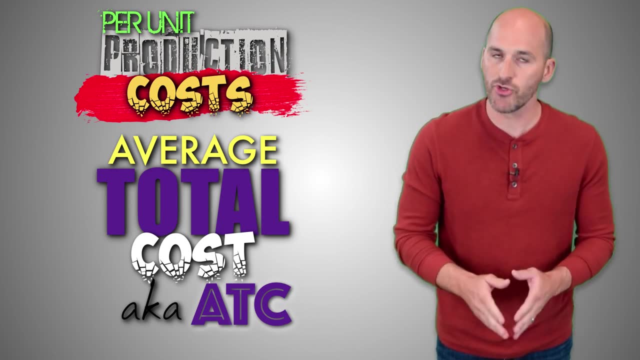 cost of production and divide it by total product. Average total cost tells the firm the combined cost of both fixed and variable resources per unit of output produced. In other words, it tells the firm the total cost of production per unit of output. To calculate the average total cost per unit, we simply need to take the total cost of production. 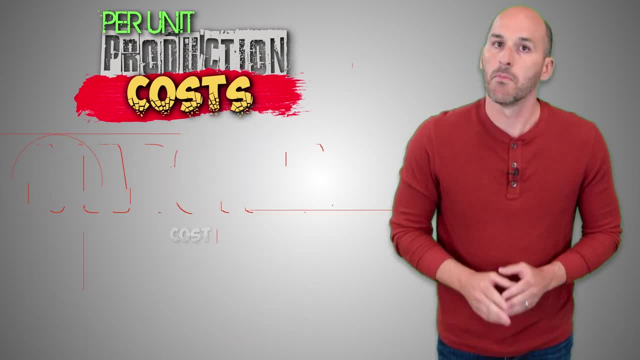 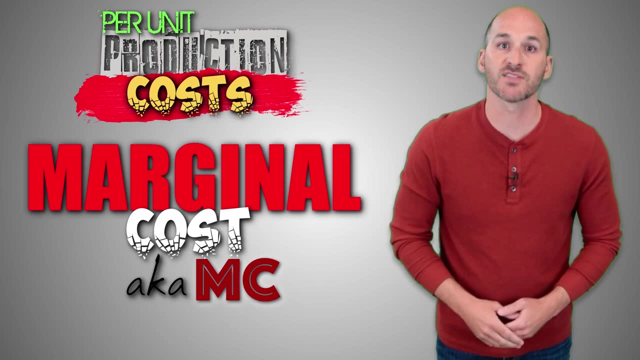 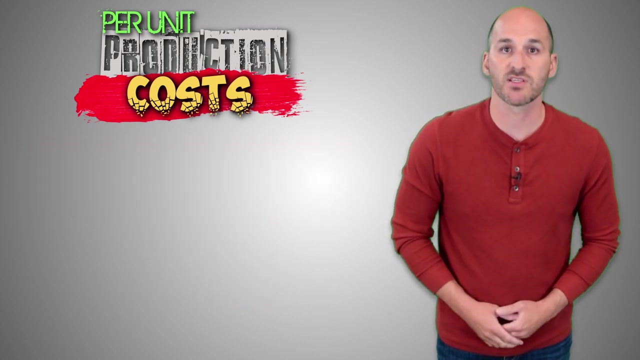 and divide it by total product. Marginal cost is the cost of producing each additional unit of output. In other words, by how much will total cost increase with the production of each additional unit of a good or service? To calculate the marginal cost of each unit of output, we simply need to take the change. 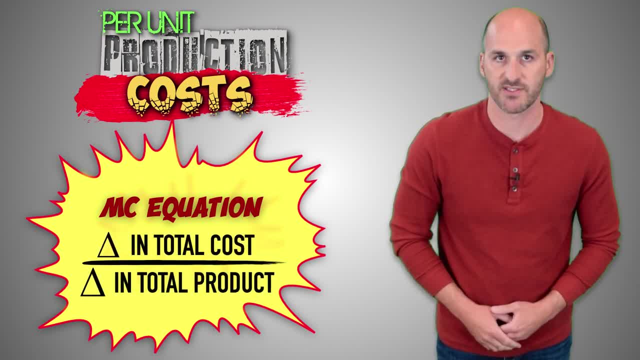 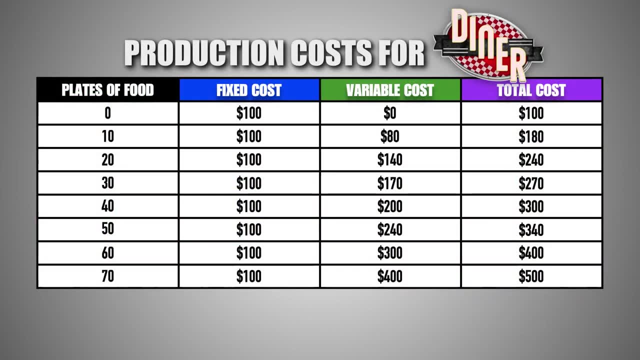 in total cost and divide it by the change in total product. Let's take a closer look at calculating per unit production costs. Let's go back to that small diner in your hometown. Here we can see the production cost that we calculated earlier. We can use the fixed cost, variable cost and total cost of production at each level. 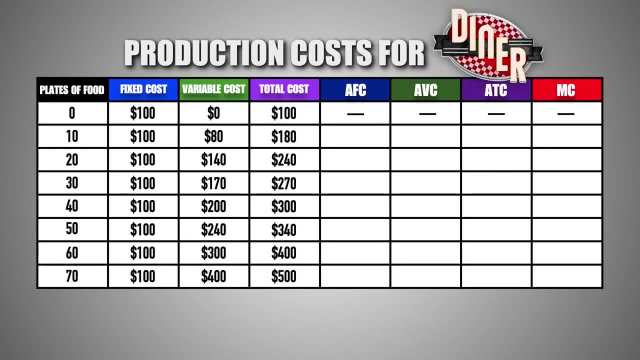 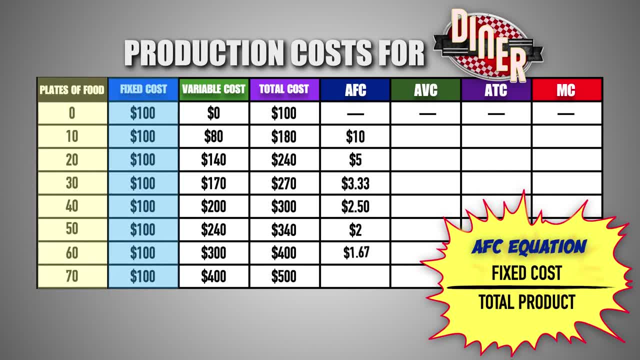 of output. to calculate the per unit production costs for the firm, Let's start with the average fixed cost. We can divide fixed cost by the total product at each output level to find the average fixed cost per unit. Next let's calculate average variable cost. 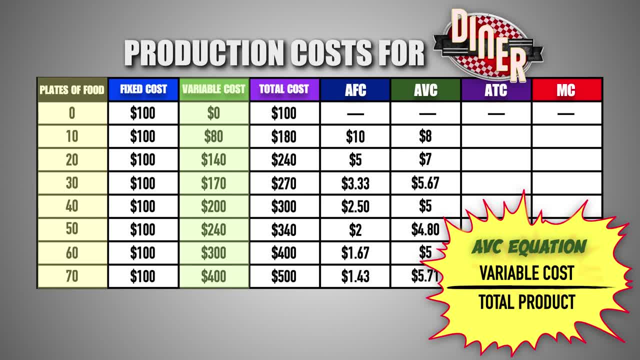 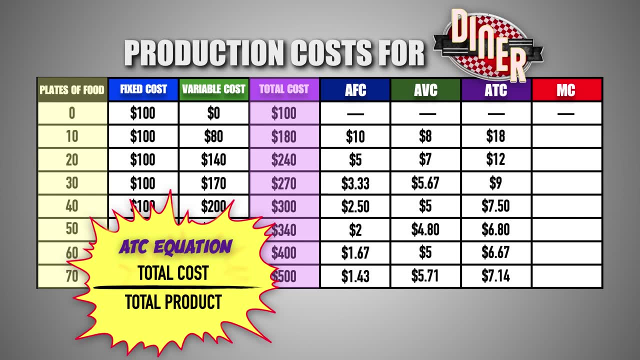 We can divide variable cost by the total product at each output level to find the average variable cost per unit. Now let's calculate average total cost. We can divide total cost by the total product at each output level to find the average total cost per unit. 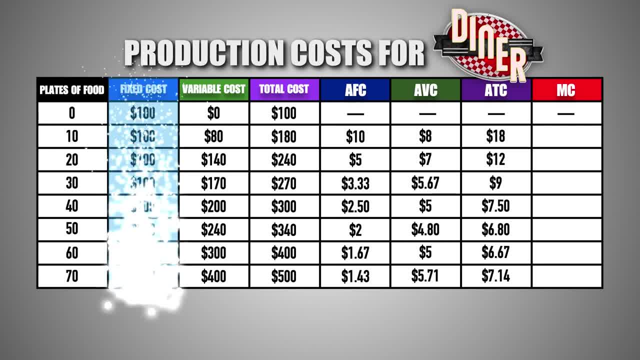 However, because total cost is the sum of fixed cost and variable costs, total cost can also be found by adding the average fixed cost per unit to the average variable cost per unit. And lastly, let's calculate marginal cost At each output level. the diner increases its total product by 10 meals. 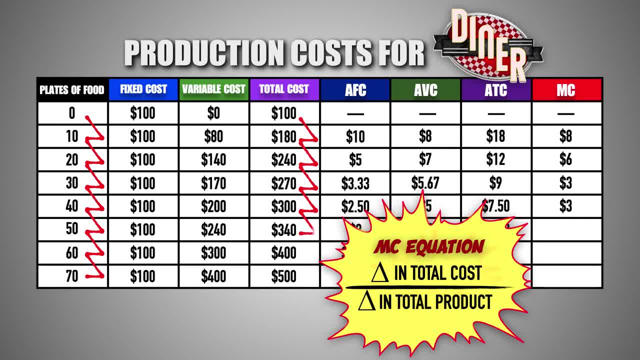 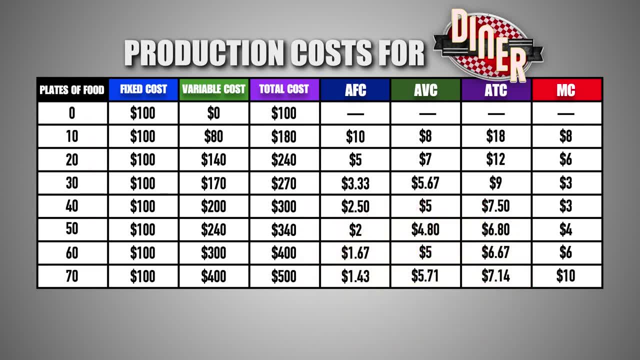 As a result, we can divide the change in total cost at each output level by 10 meals to find the marginal cost of producing each additional meal. Notice several things. Each of these sums represents the fixed cost, variable cost and total cost of producing. 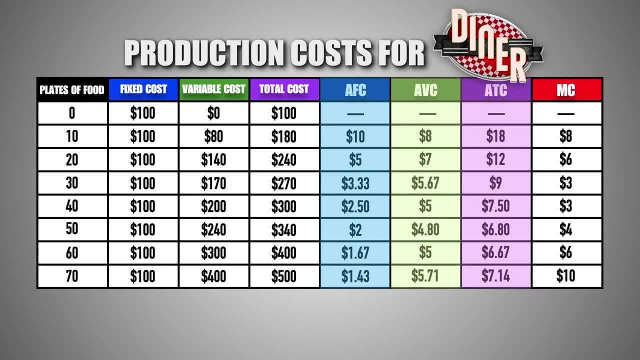 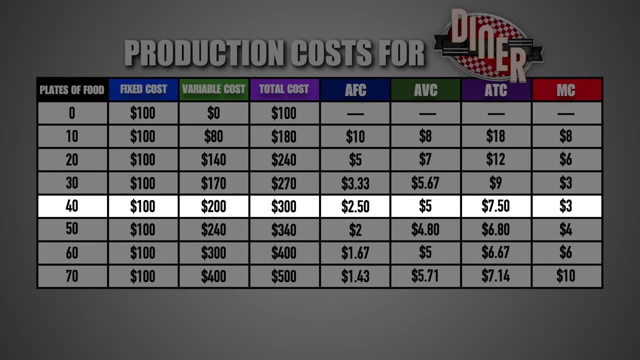 each meal at every output level. In order to cover these production costs, the diner must sell each meal at a price that is equal to or greater than the production cost per unit. For example, when producing 40 meals, the average fixed cost of producing each meal. 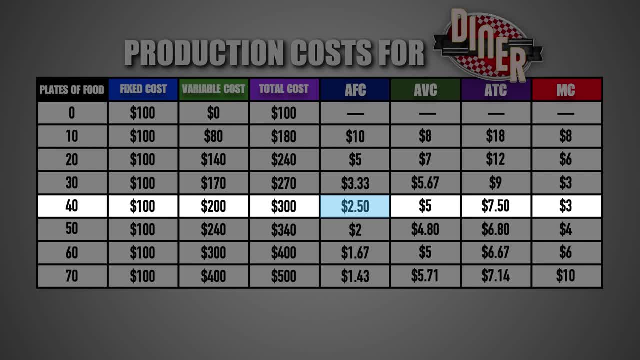 is $2.50.. In order to generate a enough revenue to cover their fixed production costs, the diner must sell each meal at a price of $2.50 or higher. When producing 60 meals, the average variable cost of producing each meal is $5. 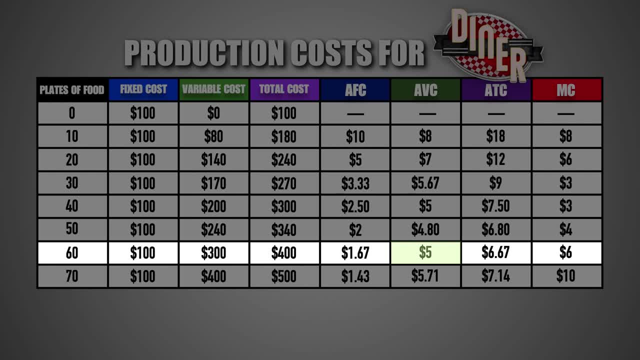 In order to generate enough revenue to cover their variable production costs, the diner must sell each meal at a price of $5 or higher. When producing 50 meals, the average total cost of producing each meal is $6.80.. In order to generate enough revenue to cover their total production costs, the diner must 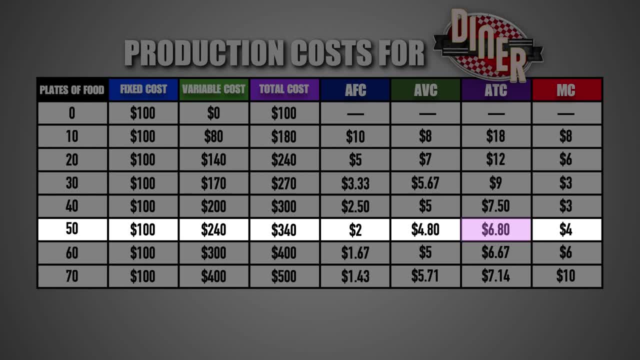 sell each meal at a price of $6.80 or higher. Also, notice that the fixed cost per unit gets smaller as total product increases. This is because, as production increases, fixed production costs, which remain constant, are divided among more and more units of output. 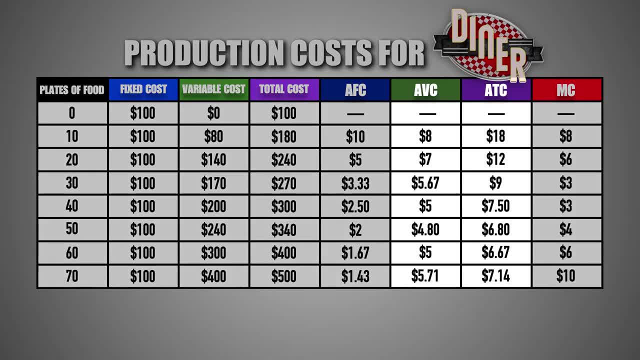 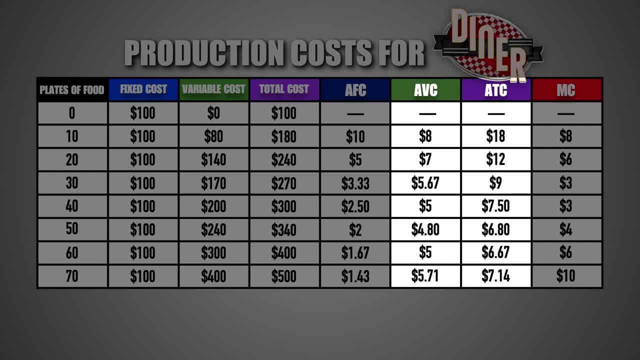 This is because, as production increases, fixed production costs, which remain constant, are divided among more and more units of output And, lastly, notice that the average variable cost and the average total cost initially decrease and then increase as total product rises. This is due to the law of diminishing marginal returns. 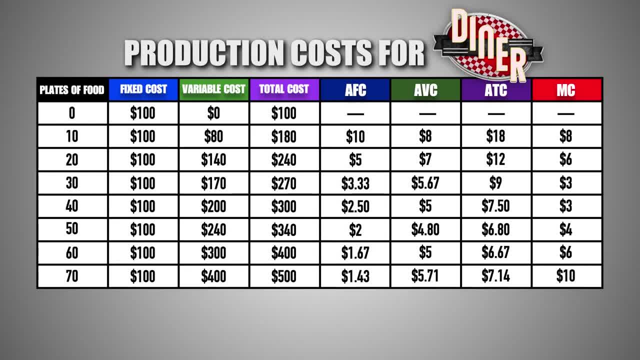 Initially, variable resources are more productive for the firm, meaning each unit of output they produce has a lower variable cost. Then, as diminishing return sets in, each additional variable resource is reduced to $5.50.. This means that each variable resource is less productive than the last, causing the 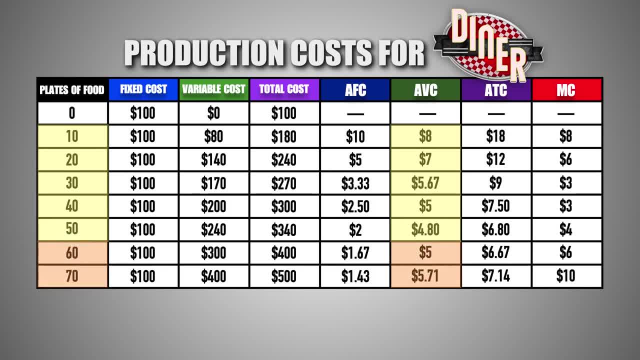 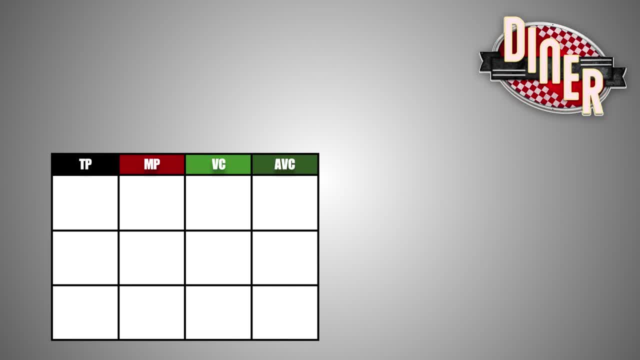 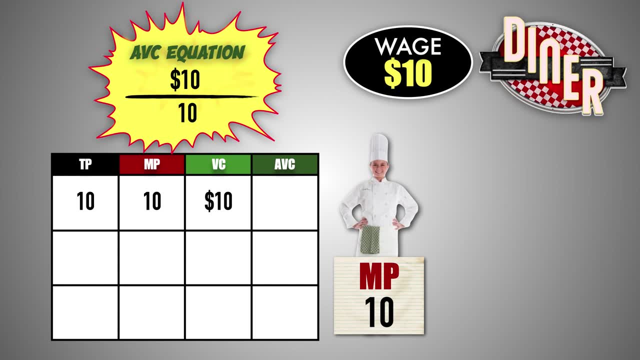 variable cost per unit of output to increase again. Let's put it this way: Suppose the diner hires three workers and the only variable cost is the hourly wage of $10 paid to each worker. If the first worker can produce 10 meals, each meal has an average variable cost of